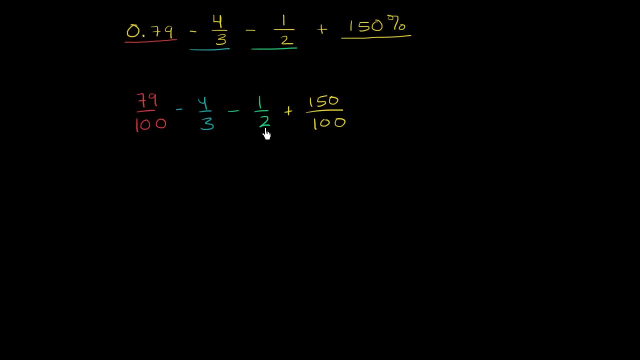 So 100 is actually the least common multiple of 100 and 2.. So we really have to just find a least common multiple between 100 and 300. And that's just going to be 300. There's no other common factors between 100 and 3.. 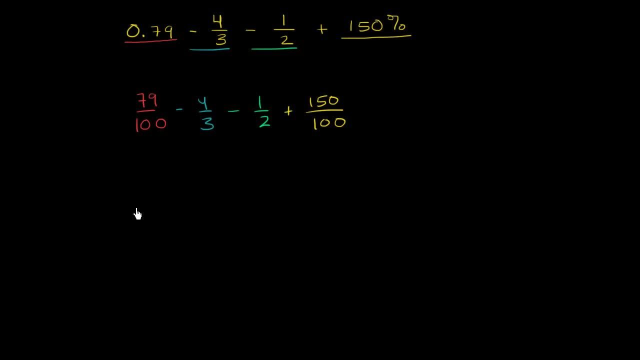 So let's write all of them with 300 as the common denominator. So let me do this in this reddish color. So 79 over 100 is the same thing. If I were to write it over 300, to go from 100 to 300. 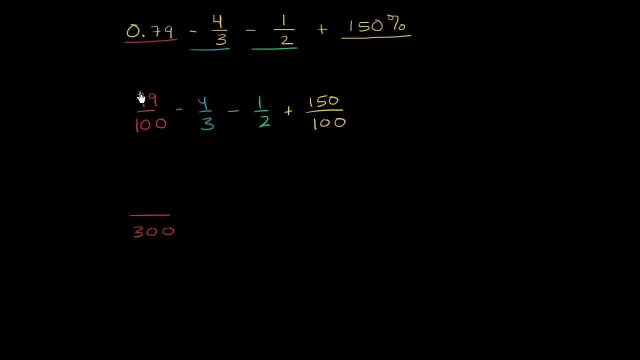 in the denominator, I'm multiplying by 3.. So I have to multiply the numerator by 3 as well. So I'm going to multiply by 3 as well. Let's see, 80 times 3 would be 240.. So it's going to be 3 less than that. 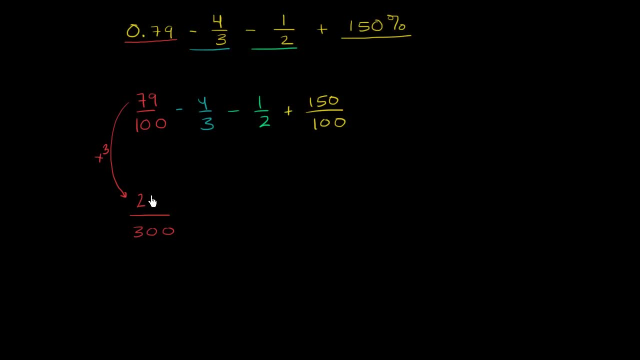 So 240 minus 3 is 237.. Now 4 thirds. Well, to get the denominator to be 300, we have to multiply the denominator by 100.. So we have to multiply the numerator by 100 as well: 1 half. 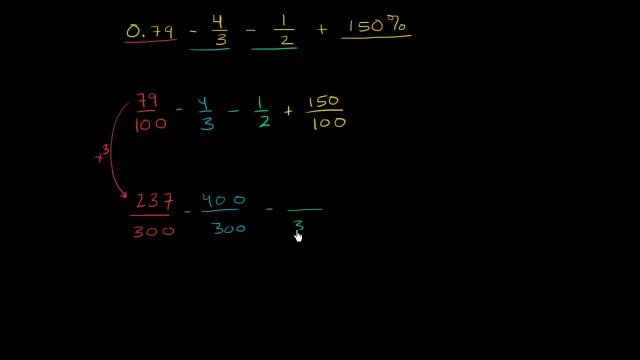 If our denominator is 300, we multiply the denominator by 150 to go from 2 to 300. So we have to multiply the numerator by 150. And then finally, 150 over 100.. Well, we're multiplying the denominator by 3. 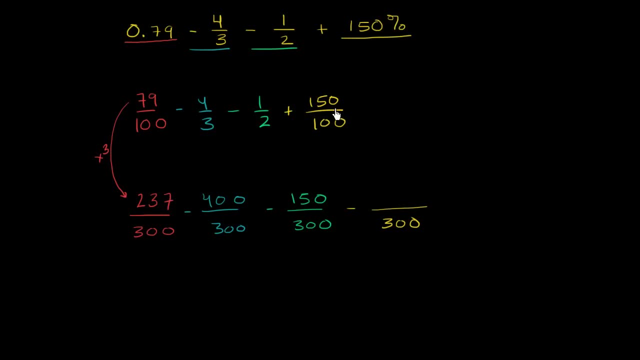 to get to 300, to go from 100 to 300. So we have to do the same thing in the numerator. So 3 times 150. So 150 is 450.. So now we have the same denominator And we can now add our numerator. 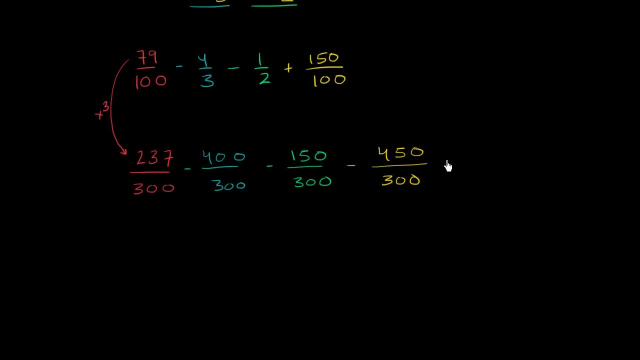 So this is going to be equal to- actually- I could just do it right over here on the right-hand side- This is going to be equal to some stuff over 300.. So it's going to be 237 minus 400 and minus 150. 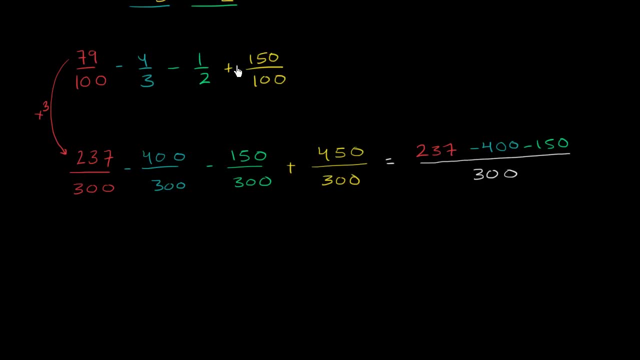 And this actually should be a plus right over here. This should be plus 450.. And so let's see if we could simplify this a little bit. We're subtracting 400, and we're subtracting 150. So these two would be the same thing as subtracting 550.